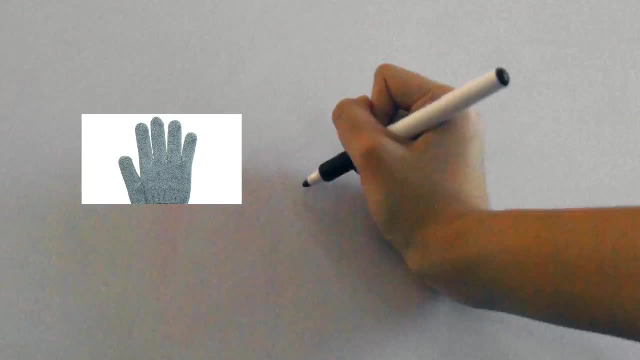 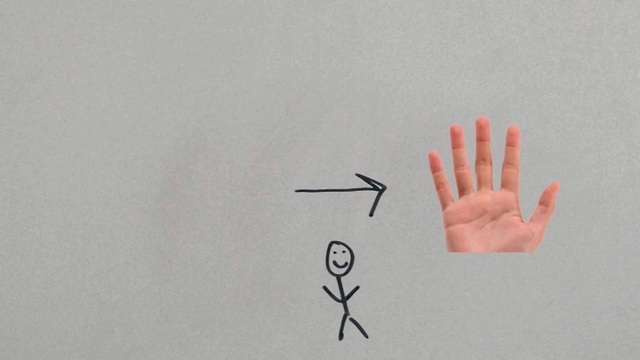 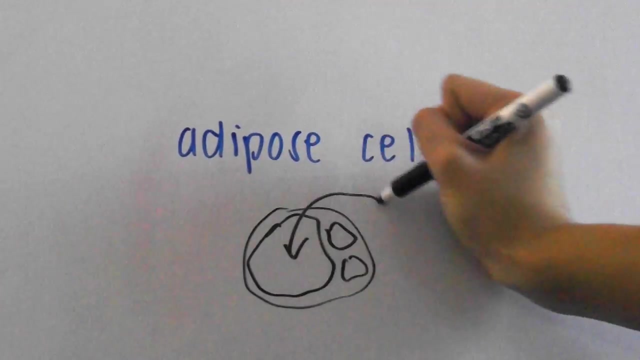 makes sense. For example, the structure of a glove is the shape of a hand, and its function is for the person to wear the glove so his or her hand can be protected. The same thing goes for cells. One type of cell we'll look at is a fat cell or one in adipose tissue. It has a large storage area, while 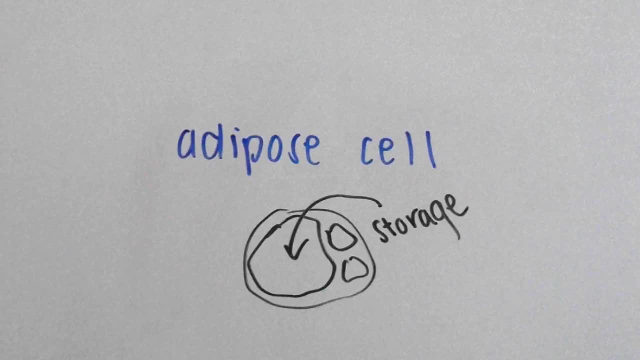 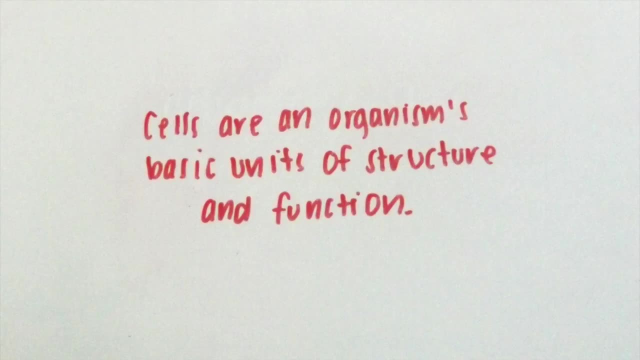 its nucleus and cytoplasm are pushed to the side so it can store all of its energy. This also goes hand in hand with the next theme. Cells are an organism's basic units of structure and function. We just talked about that, but it might be good for you to brush up on the cell theory. 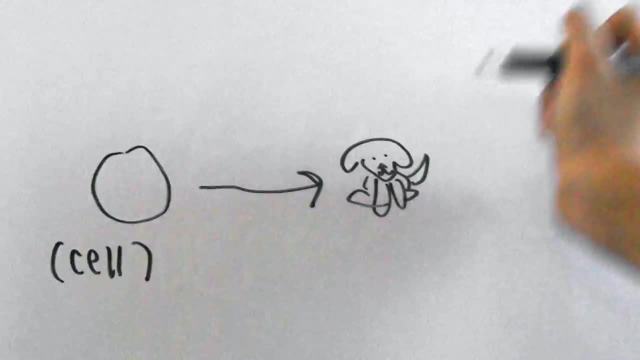 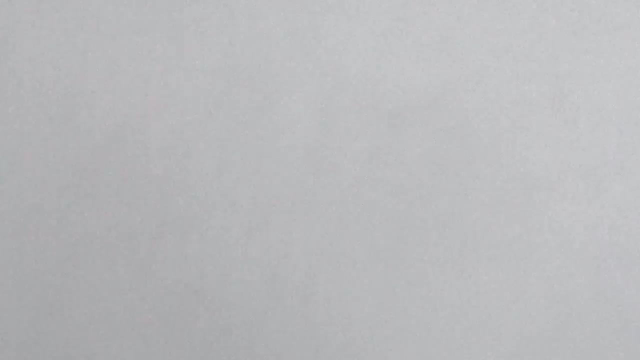 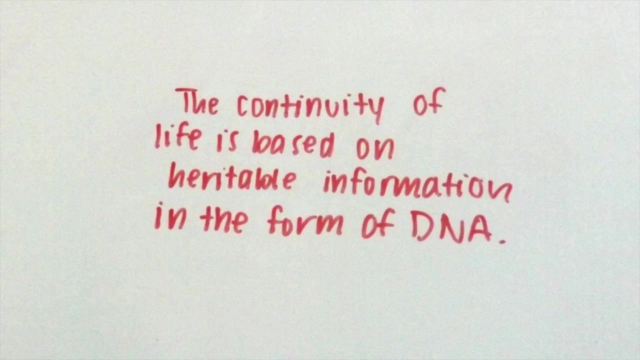 First of all, cells are the basic unit of function in an organism. Second, all living things are made of cells. and finally, only existing cells can make new cells. On the topic of cells making new cells, the next theme says that the continuity of life is based on heritable. 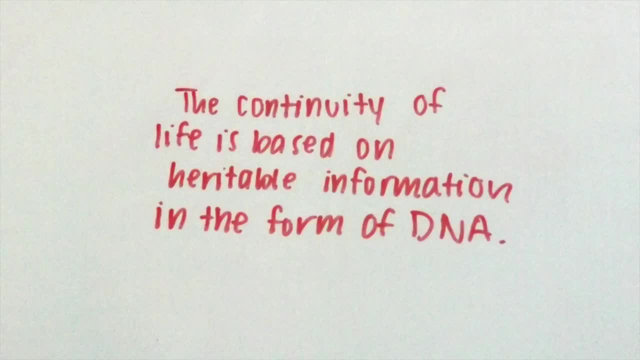 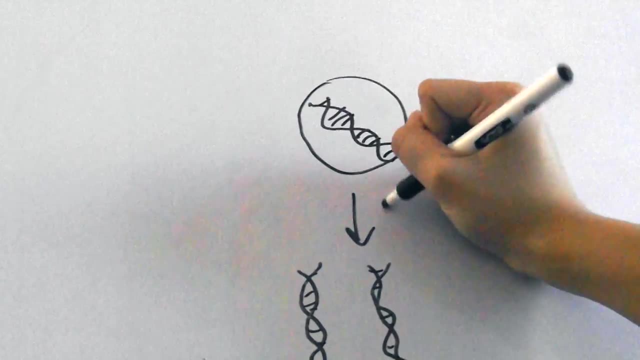 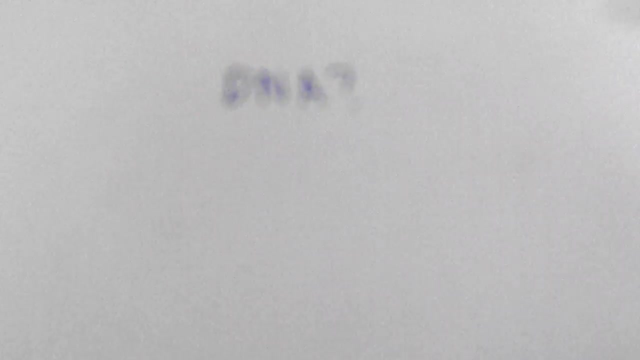 information. This is information in the form of DNA. This is saying that DNA, the genetic material of most organisms, is used to pass on genetic information to all offspring. Some organisms actually use RNA, which is another nucleic acid, to pass on genetic material, but we won't get into that until later. 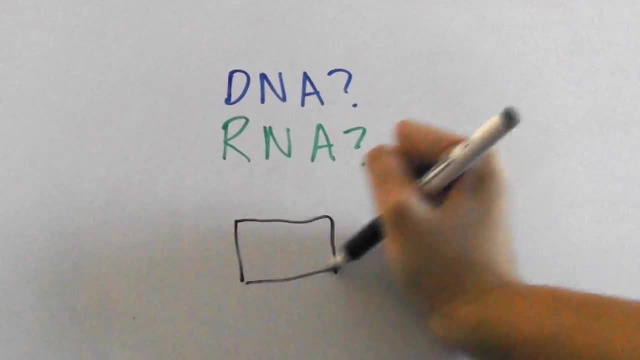 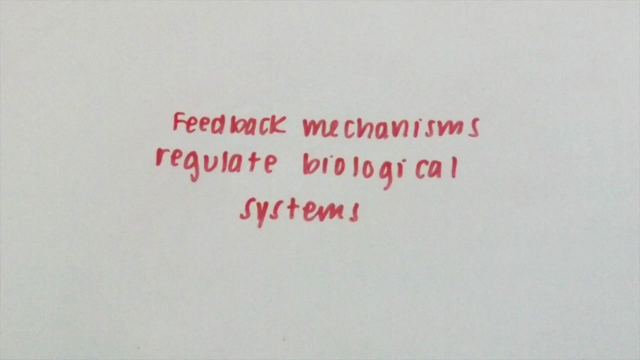 in the course. The last theme is that feedback mechanisms regulate biological systems. You may have seen me explain this in my other video, the four big ideas of APS. The first is that the body of a cell is a cell. The second is that the cell is a cell. The 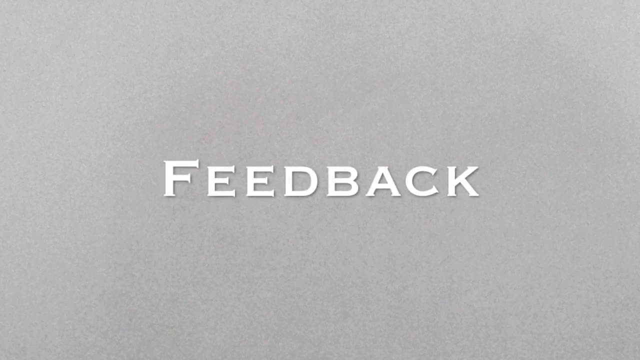 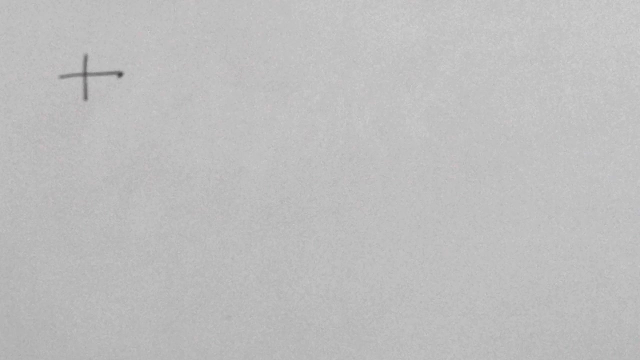 biology. but in case you haven't, I'll tell you right now that there are two types of feedback: positive and negative. Here are some analogies for both. For positive feedback, think of your favorite food, the most delicious thing you have ever eaten in the world. Okay, now here's a. 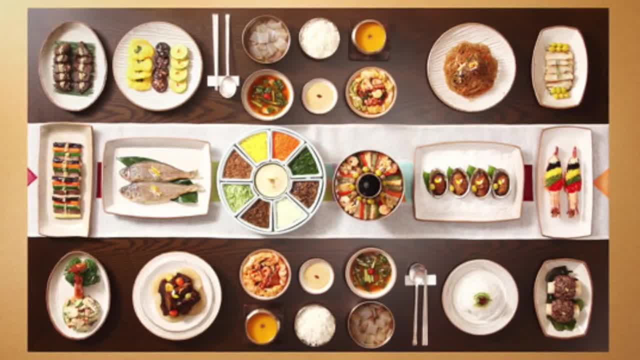 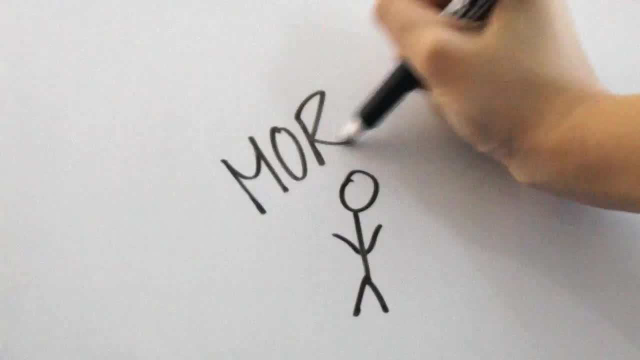 no-brainer. Would you stop at just one bite of this glorious meal? No way, You would keep eating and eating. and the same idea goes for positive feedback. Even though a lot of a product may be accumulating, the process that makes the product keeps going and going, so that it amplifies the 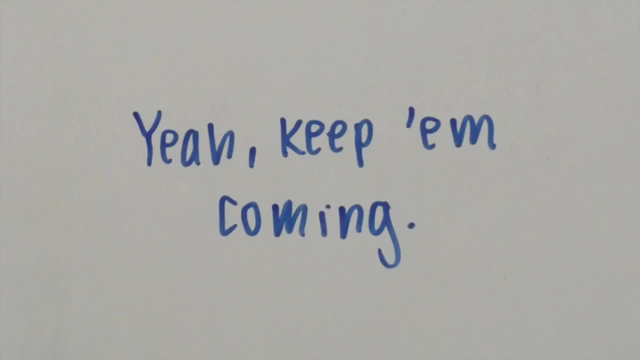 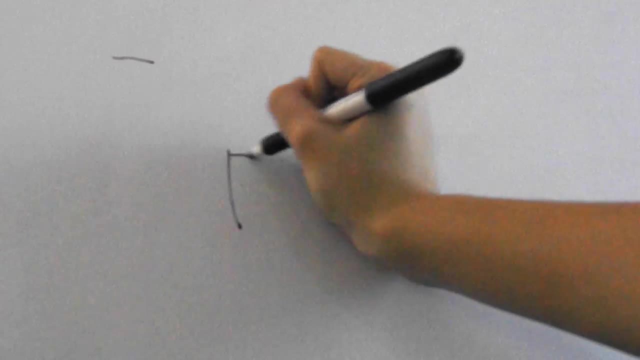 quantity of the product. Negative feedback is the opposite. Once there is too much of a product, the body stops the process that is, making it so that there is not an excess of it anymore. For instance, if you were pouring water into a cup, you would stop once there would be enough.